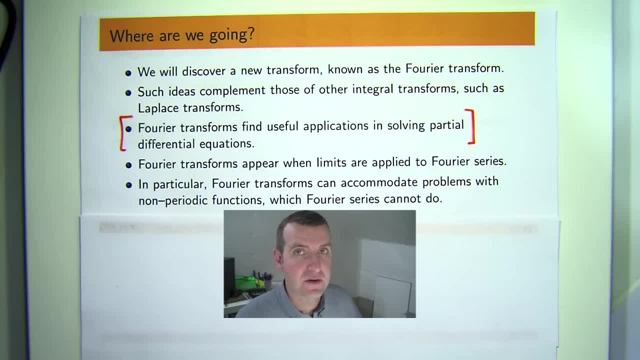 this naturally raises the question: what about non-periodic functions? And Fourier transforms can accommodate these kinds of non-periodic functions where Fourier series can't handle them. So this is something that Fourier transforms can do that Fourier series cannot do. Now I'm not going to show you the derivation or the suggestion of how Fourier transforms. 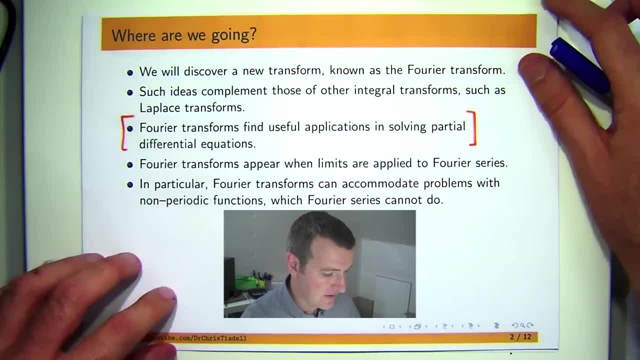 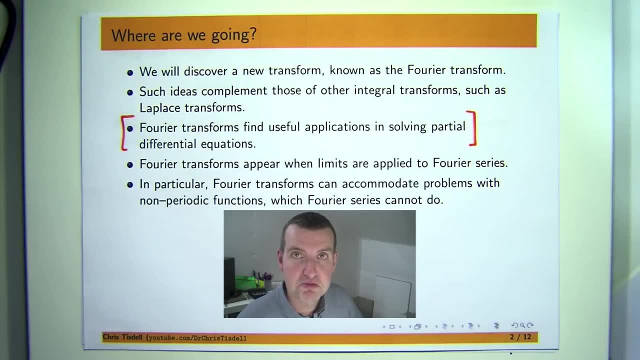 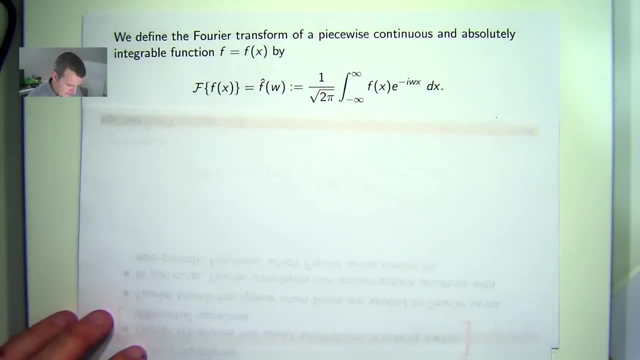 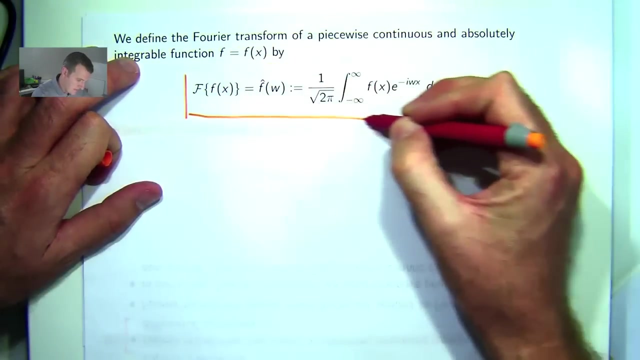 arise from Fourier series. I'll leave that for another video. But essentially what's happening is you're letting the period of the function approach infinity. What is a Fourier transform? Suppose I've got a function of one variable, f of x and 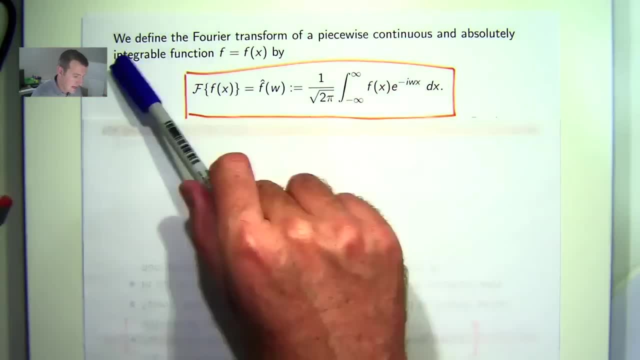 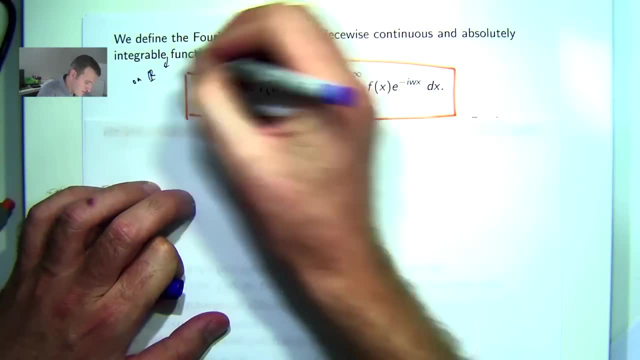 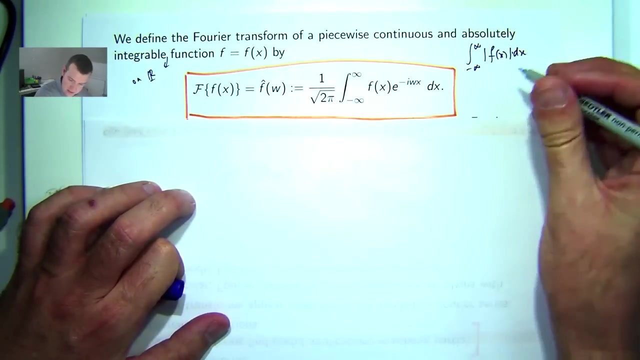 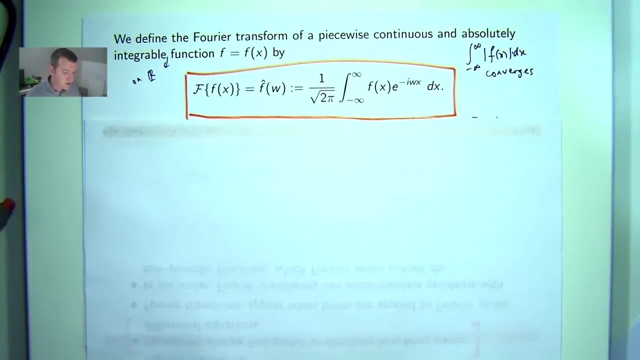 that function is piecewise, continuous, continuous and absolutely integrable on the whole real line. So by absolutely integrable I mean the following: This improper integral converges. So we define the Fourier transform of f by this integral transform. here Now, just like with Laplace transforms, there's two ways of really denoting the transform. 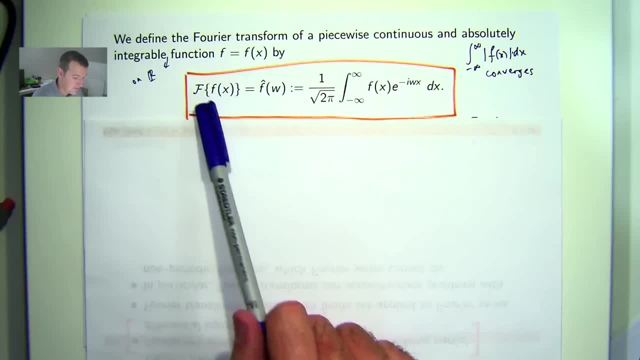 One is through this curly big F or calligraphic F. The other is through this f hat. Now, this particular notation emphasises the dependency on w. If you look over here, your dummy variable is x. You've got i. i squared equals negative 1.. 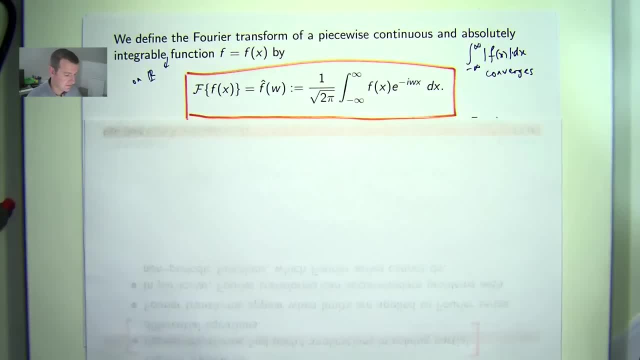 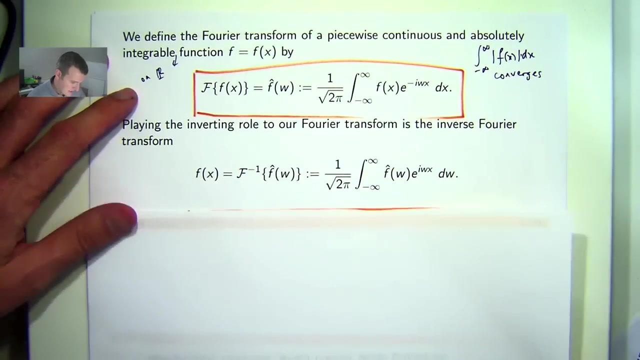 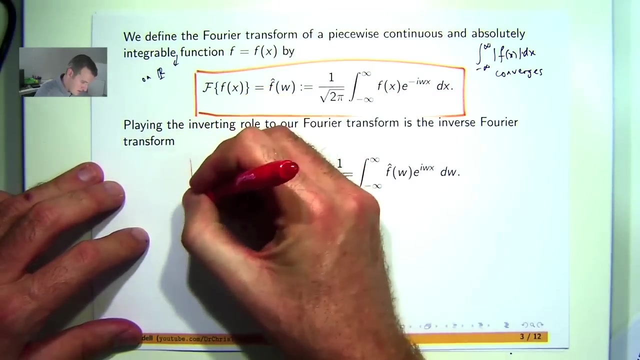 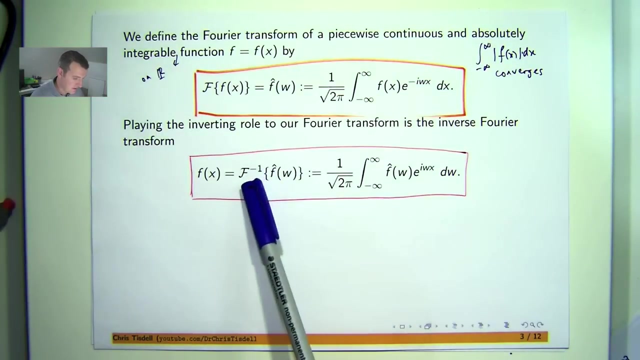 And you'll be left with some function of w here. So this notation emphasises our original function. This notation emphasises that the transform really is a function of w And there is a partner to our Fourier transform. So what could be defined through the following? 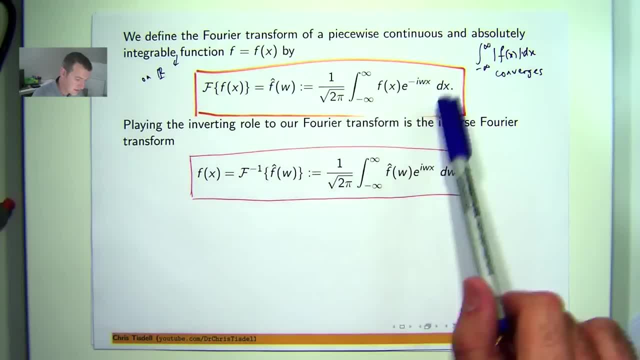 Well, we have this curly F inverse, And if you apply this curly F inverse to this, you should recover the original F of x. Now some books have different coefficients. here It's not a big deal. Almost everyone understands that. some cars here are like that. 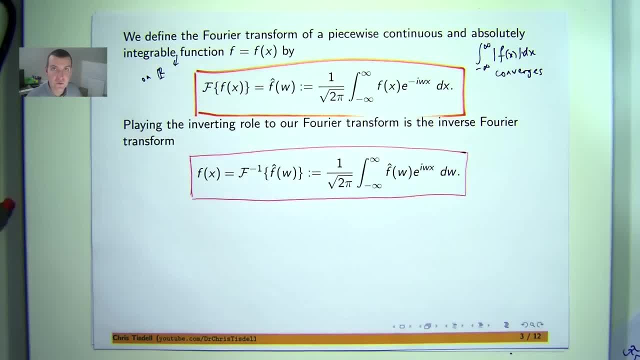 The important thing is that the product of these coefficients should equal 1 onto pi. What the point here is that all the physical coefficients, the third-쳤 points. here I have to represent at least one cevitch, But the constantρωыхme will beist. 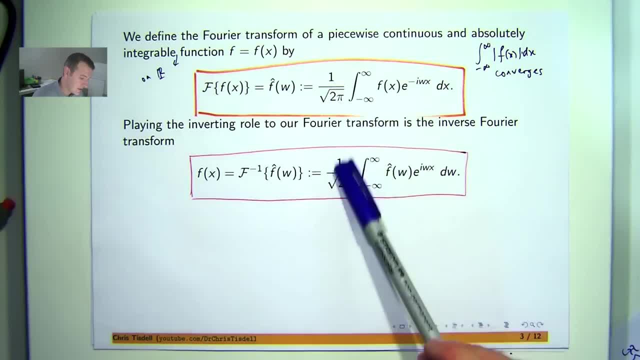 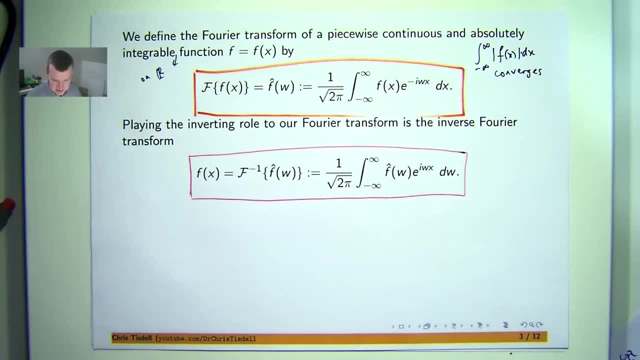 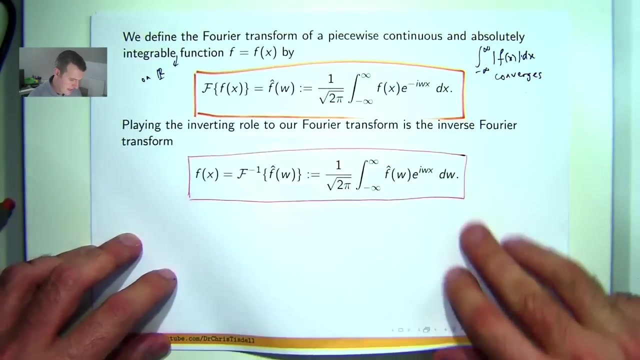 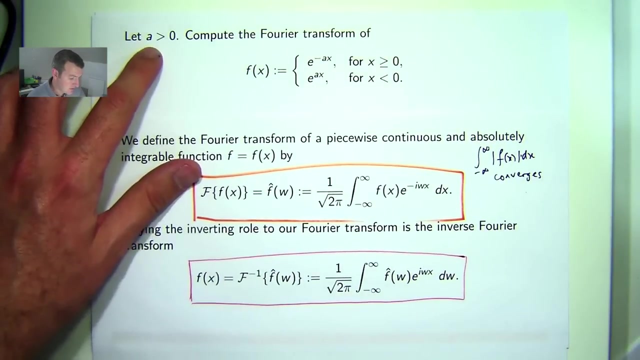 to π. So here I've got the square roots in there, just because there's a little bit of symmetry associated with each definition there. So it's not a big deal. So let's look at an example. Here's one. here We're asked to let A be a positive constant. 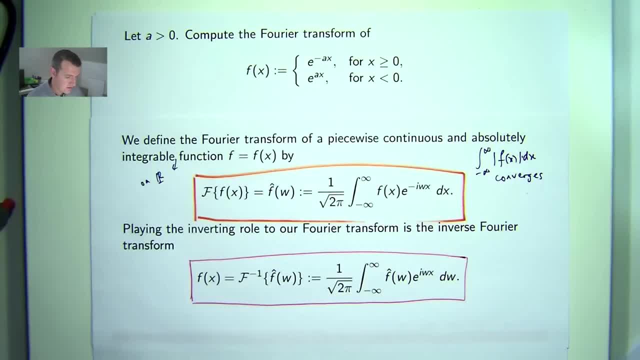 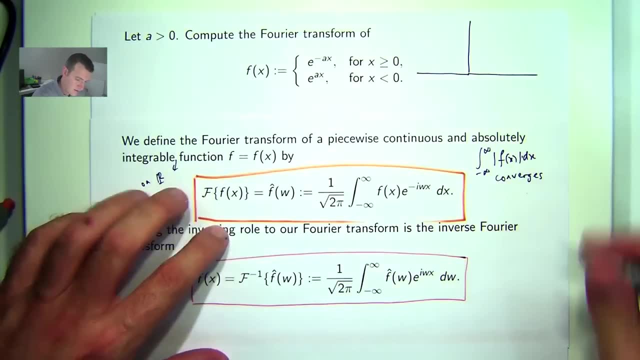 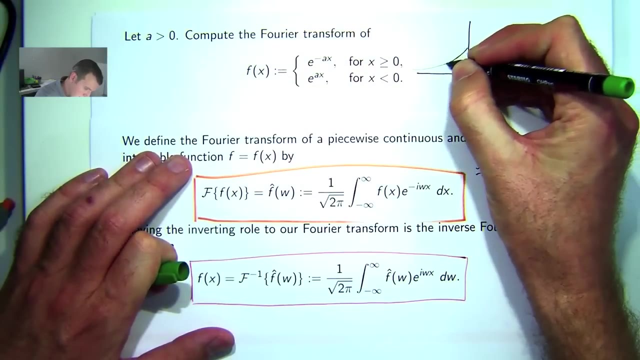 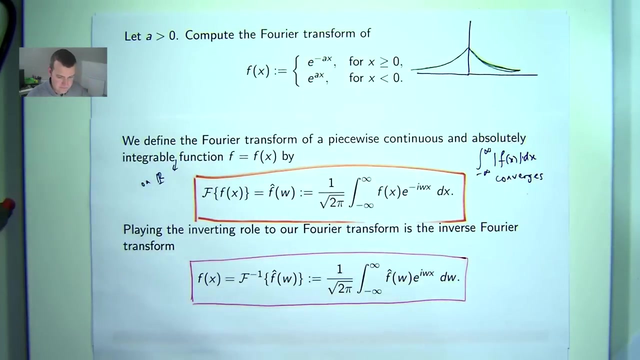 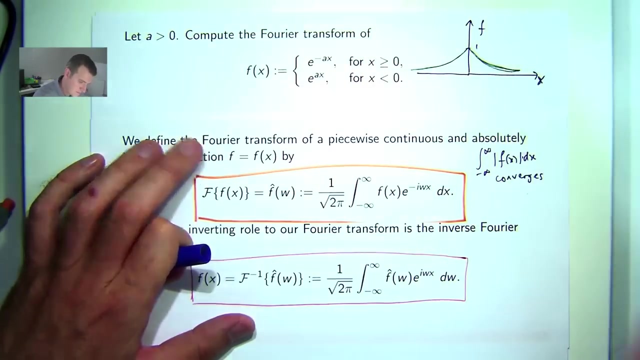 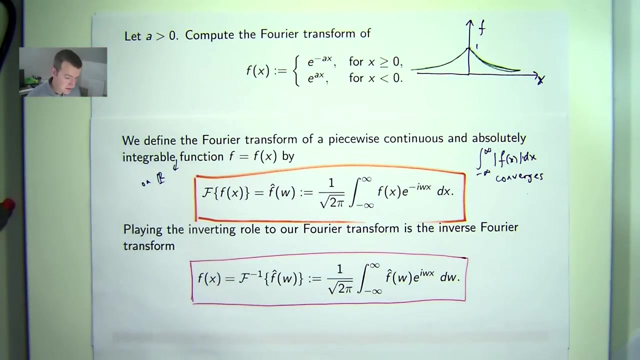 compute the Fourier transform of the following function: Okay, well, if I'm going to draw a little graph here of the function, it's going to look something like this: Okay, so it satisfies these conditions. here. Let's see if we can just apply the definition. 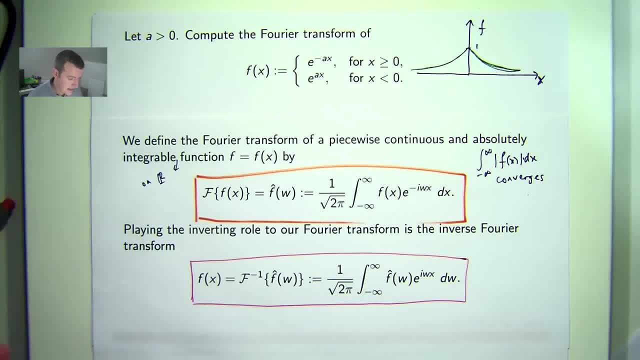 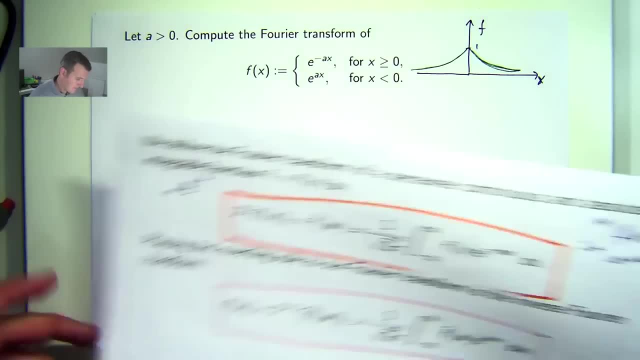 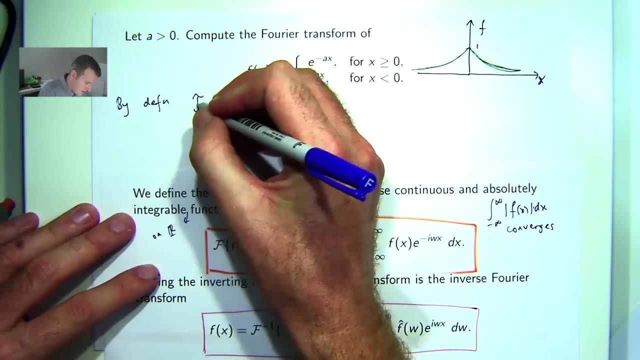 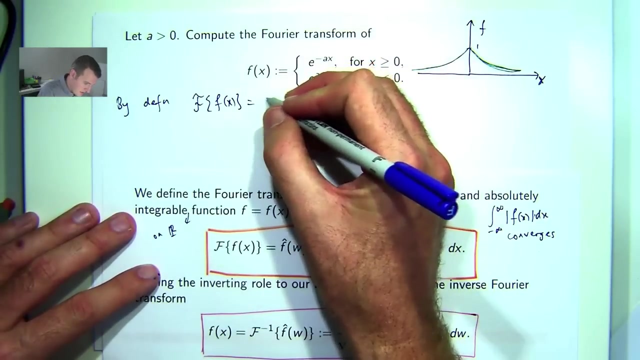 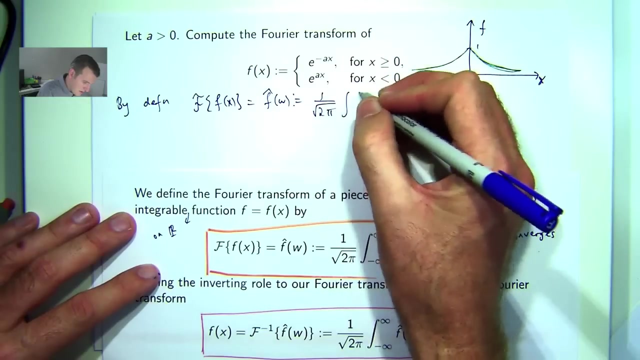 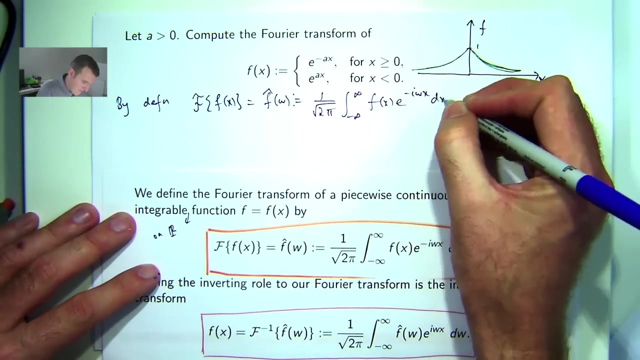 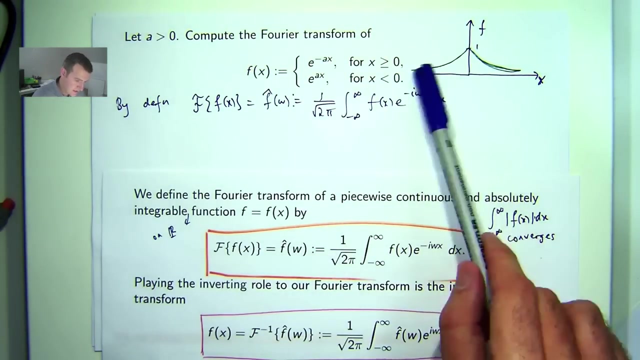 and compute the integral and the Fourier transform. Okay, so By definition, the Fourier transform of a function is just this. Okay, now our fx is defined in a piecewise way. On this interval it's defined like that, and on this interval it's defined like that. So let's break up the integral into two bits. 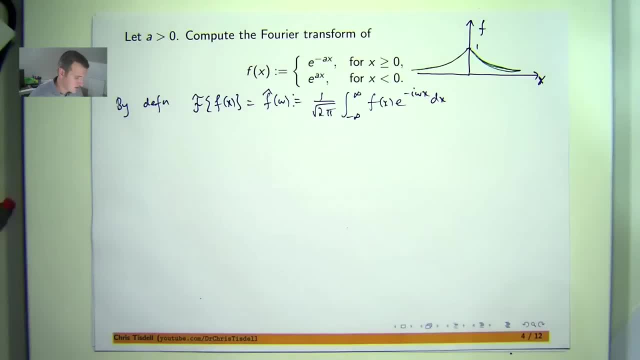 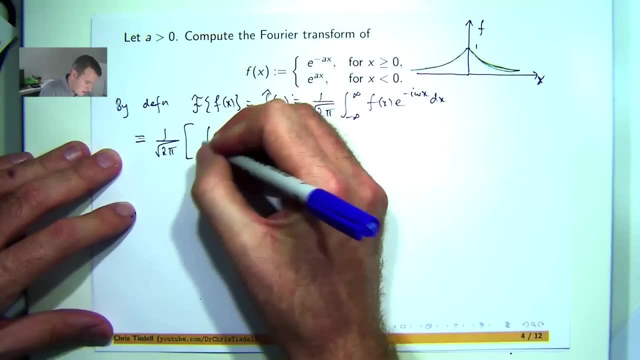 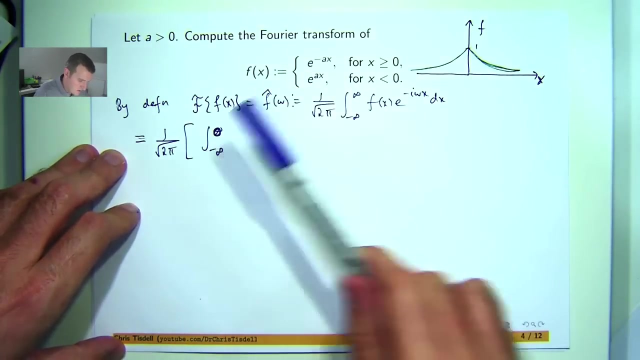 and we'll calculate both of those integrals. Okay, so, oops, Okay, negative infinity to zero, f of x on. that is the following: So it's going to be e to the ax, so I can combine it with the following: 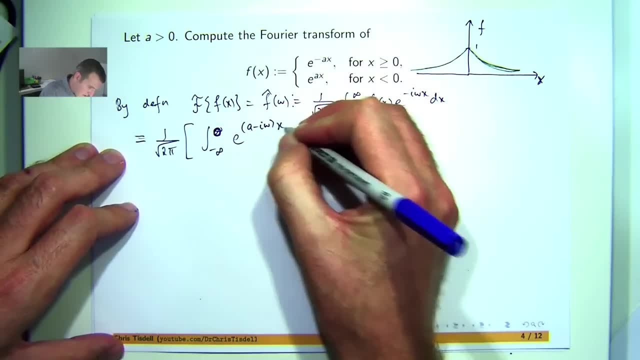 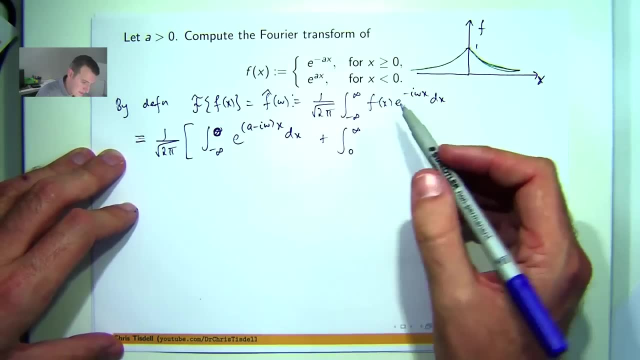 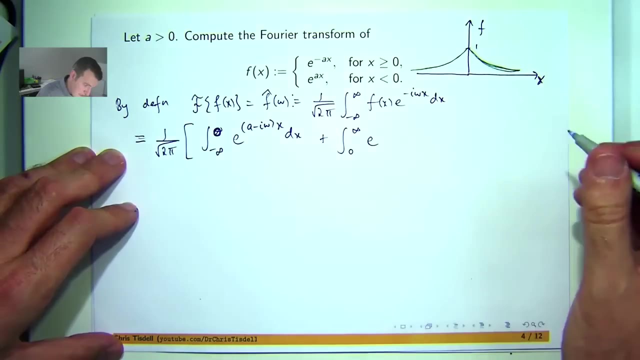 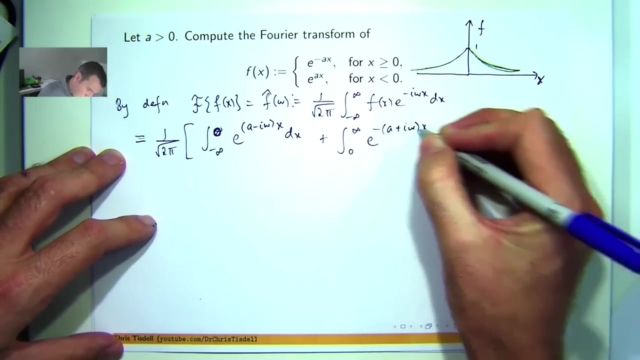 So I'll get that. And similarly, let's integrate from zero off to positive infinity, and it's going to be the following, which I can team up with my exponent there, And it's going to be something like this: Okay, so now it's just a matter of knocking over these improper integrals and then we'll be done. 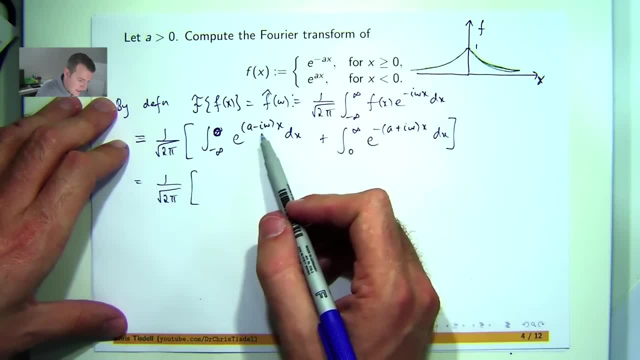 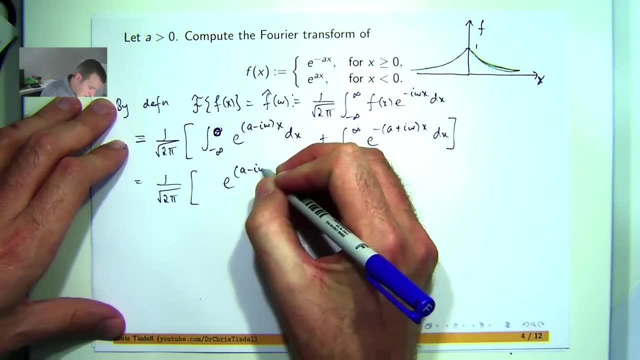 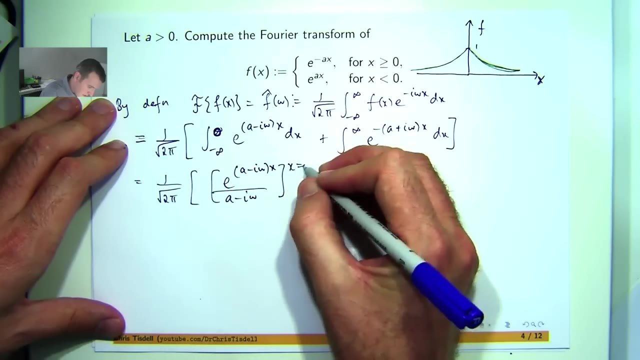 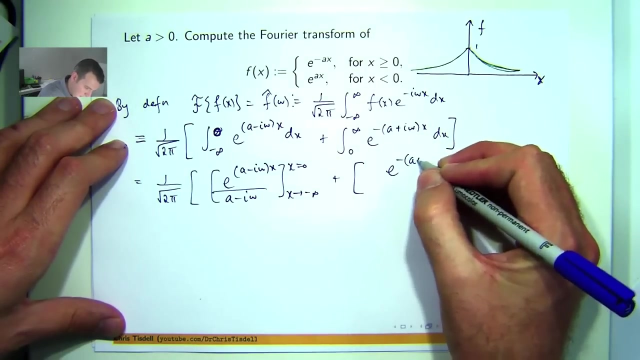 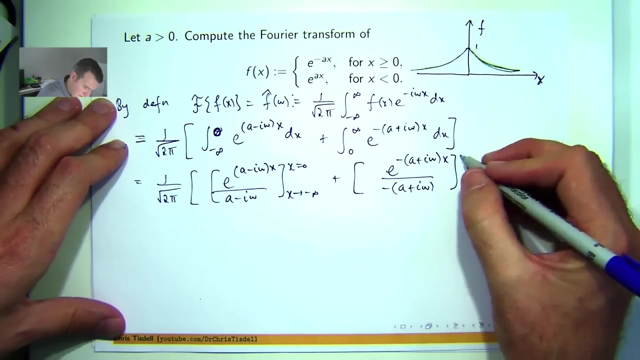 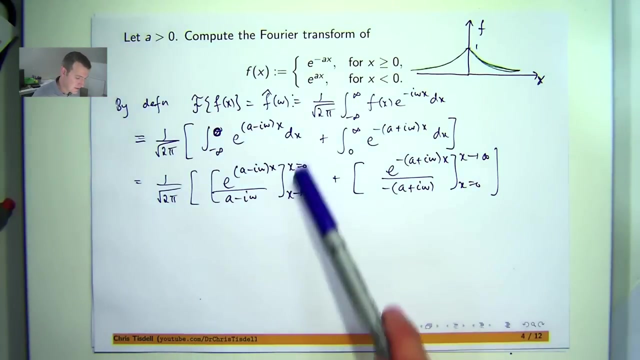 Okay, so imagine a omega and i essentially are constants, because we're integrating with respect to x, So we'll get this And same with this one. Okay, so now it's just a matter of plugging these limits in or these values in. 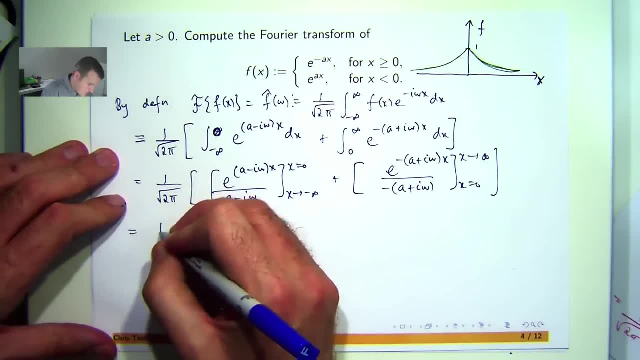 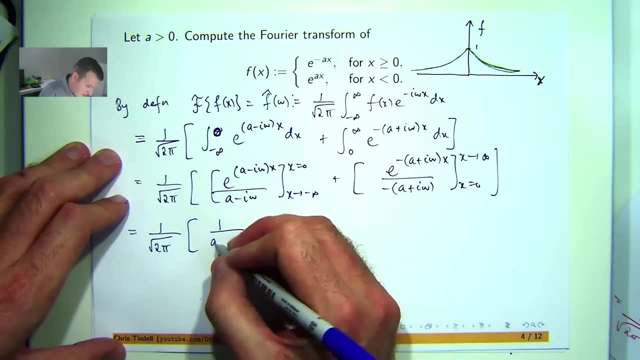 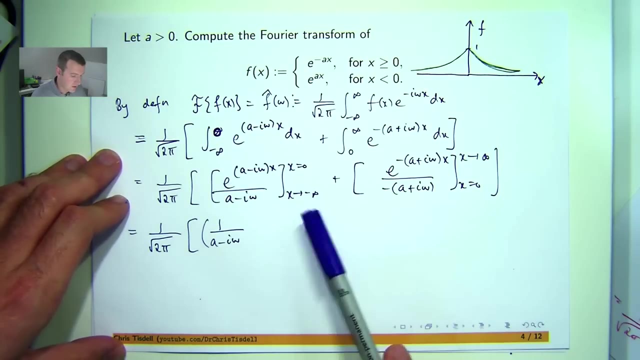 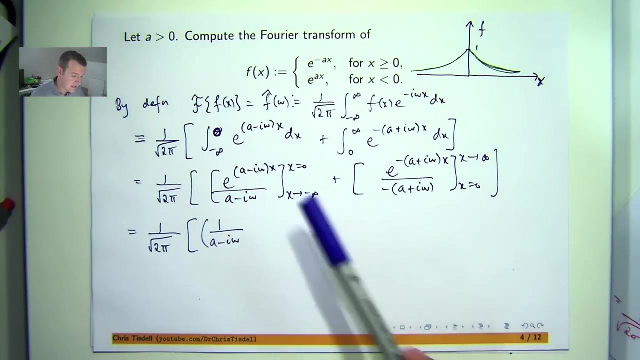 and we'll get this. And seeing what we have. Okay, so, when x equals zero, we're going to get the following: Now, as x approaches negative infinity, what's going to happen? Well, this will go to zero. Okay, essentially, what's happening there is the e to the ax. 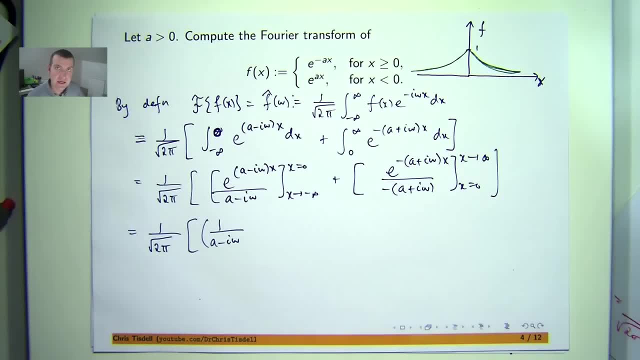 because a is positive and x is large and negative is sort of dragging everything in this term to zero. Okay, and if you want to verify that you can actually write. say e to the negative, iwx as cosine, wx minus i sine wx. 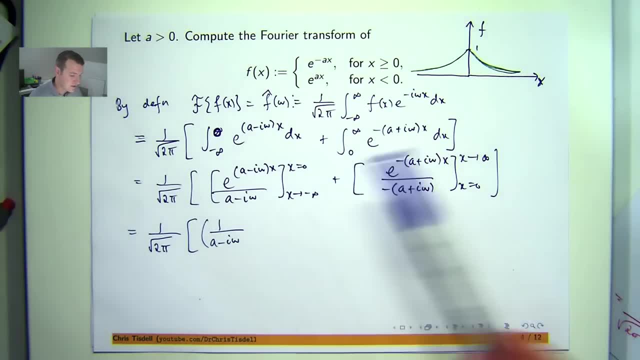 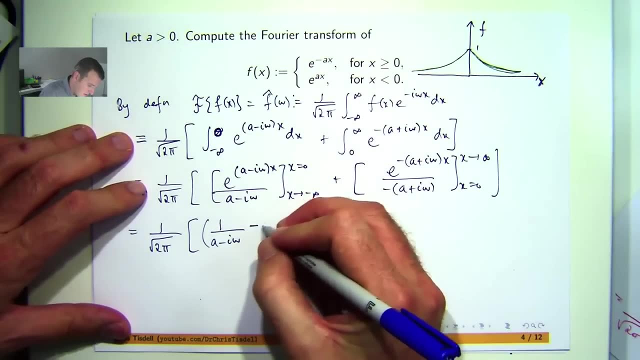 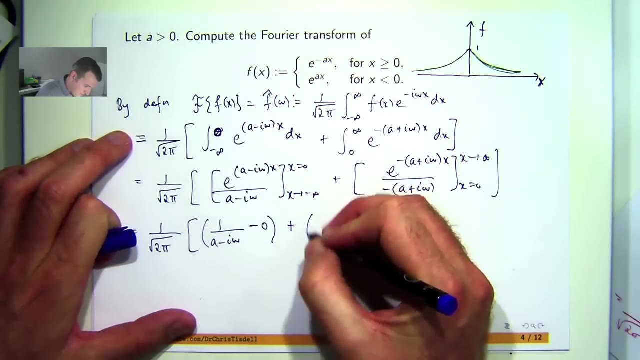 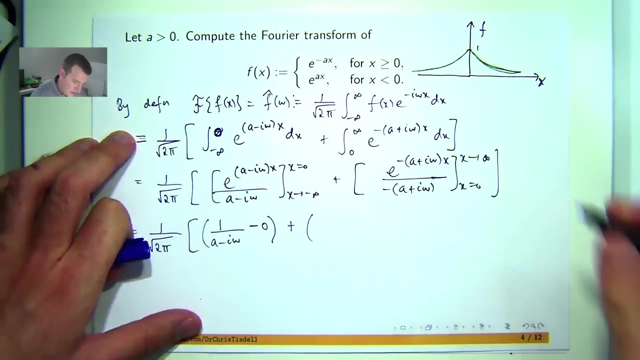 That's a bounded function. Okay, and so if I multiply by e to the ax and x goes to negative infinity, that product's going to go to zero. Okay, same over here. As x approaches positive infinity, this is going to approach zero. 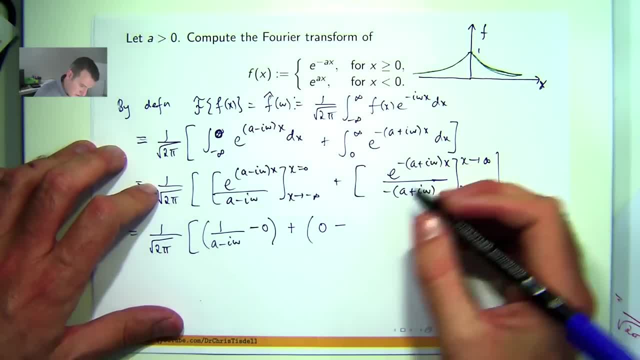 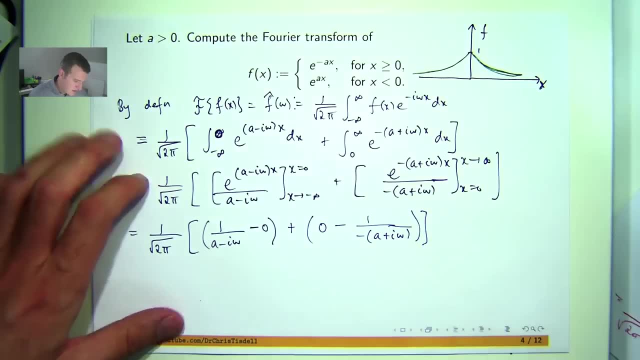 And when x equals zero, the top's going to be one, and I'm going to get something like this: Okay, Okay, so now. Okay, so now I can just sort of clean this up a bit. Okay, so I'm going to get the following: 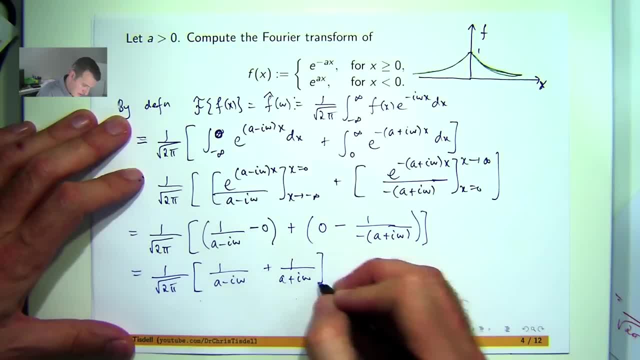 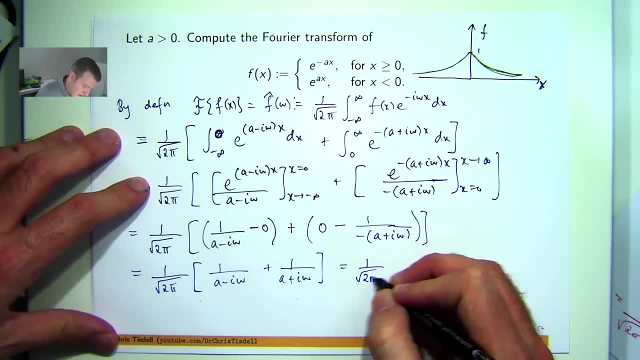 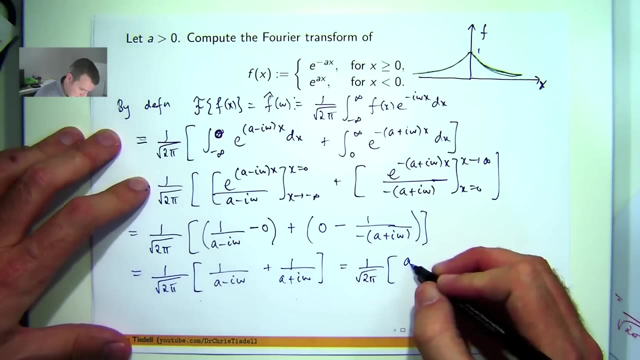 Plus. Okay, and now I can even go a bit further and get rid of the i's just by cross-multiplying: Okay. so that times that plus that, times that, all over that times that. Okay, so we're going to get some cancellation out here. 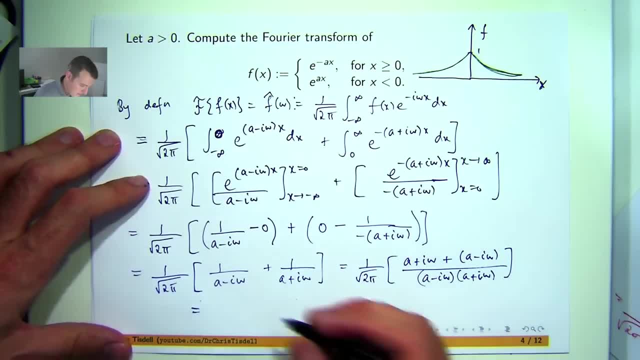 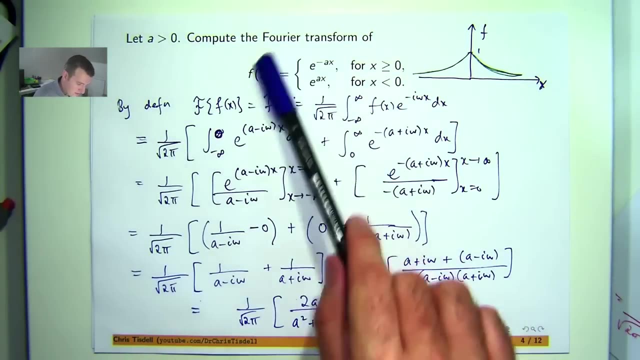 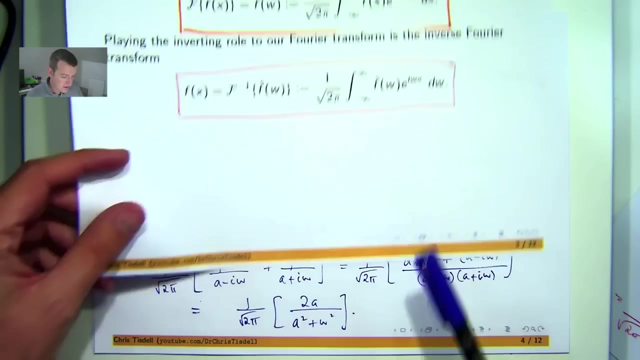 When we expand this bracket- remembering i squared equals negative one- we'll come up with the following: Okay, so the The Fourier transform of this function is this. Now, what does it mean with respect to the inverse transform? Well, the inverse transform of this is what we started with. 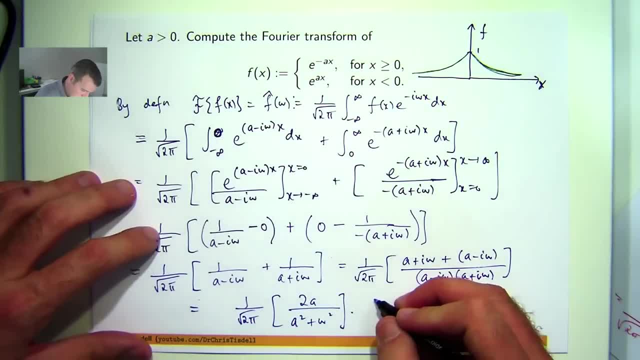 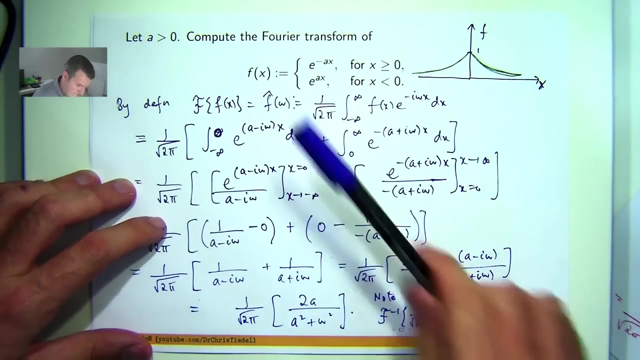 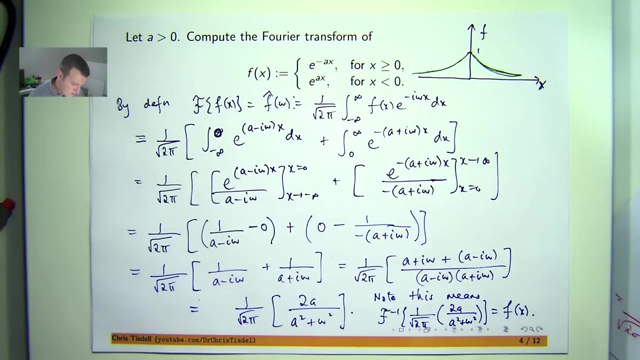 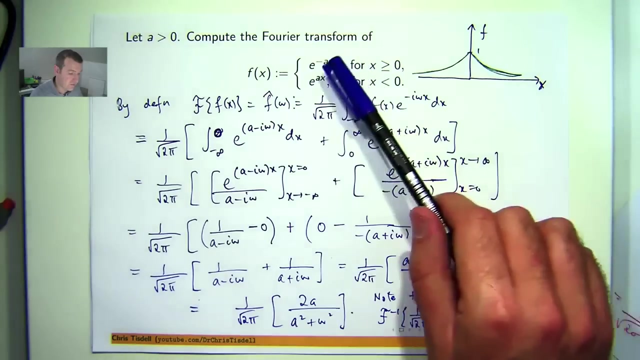 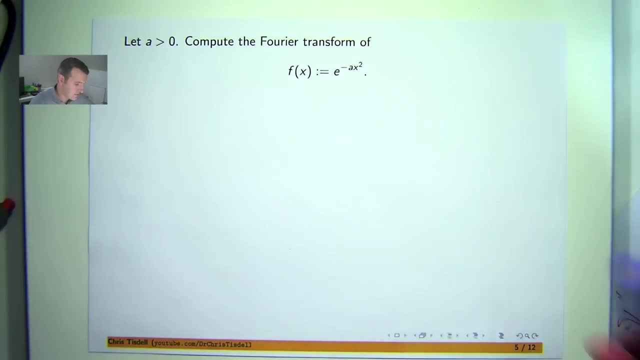 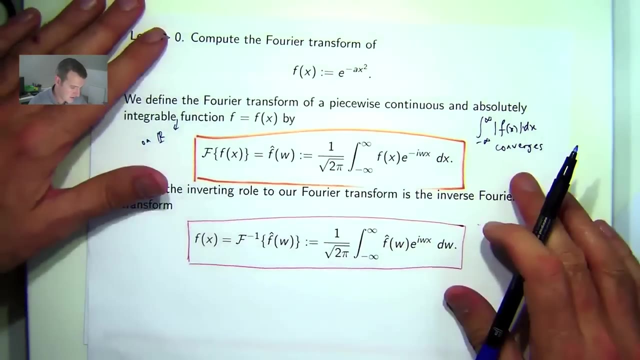 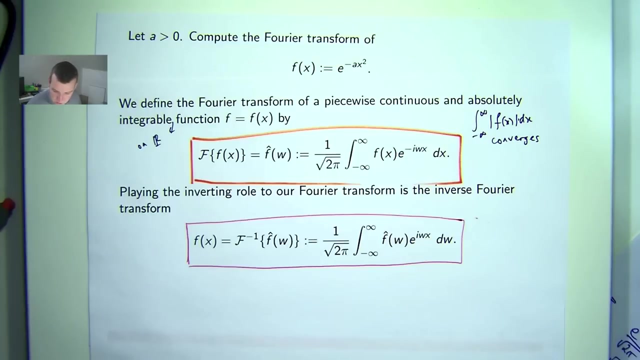 Okay, Okay, Okay, Okay, Okay, Okay. Now here we're asked to compute the Fourier transform of this particular function, and remember, this is our definition of the Fourier transform. So let's work our way through this one, and this will be a little bit more work, okay. 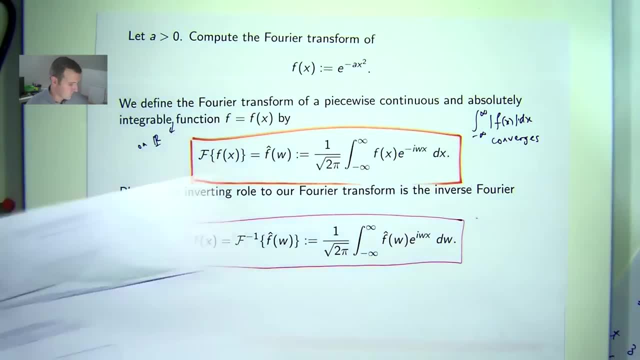 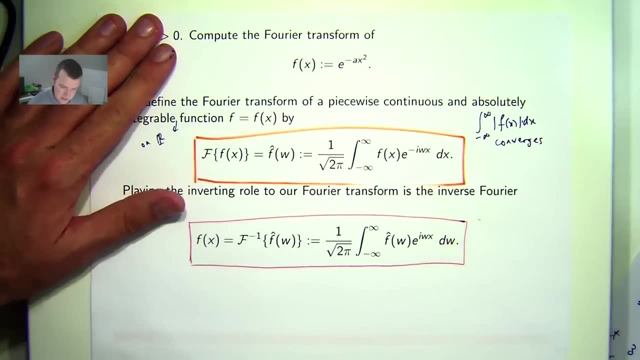 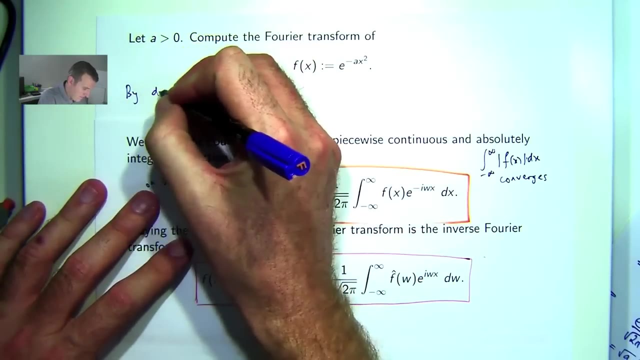 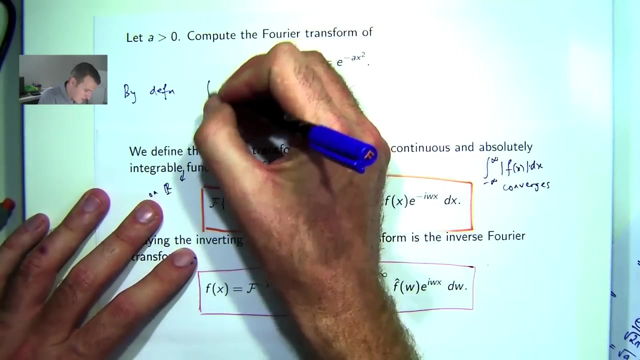 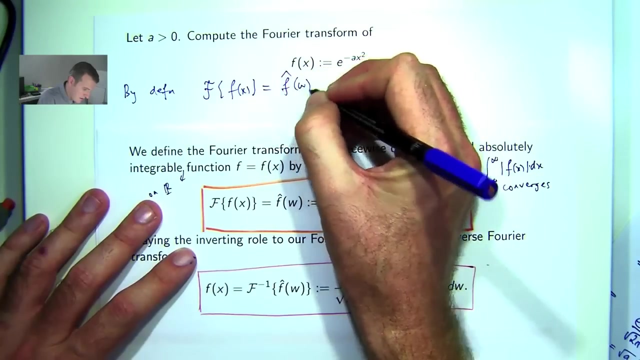 And the reason is we've got an x squared here. We did an example before where there was basically just an x up here. well, the x squared makes it a little bit more challenging. Okay, so let's use our definition. So, by definition, the Fourier transform of our given function is the following integral: 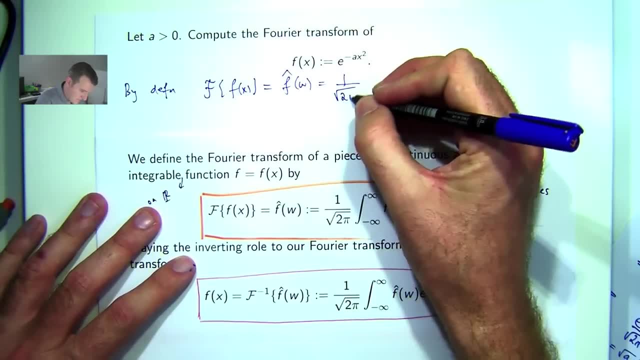 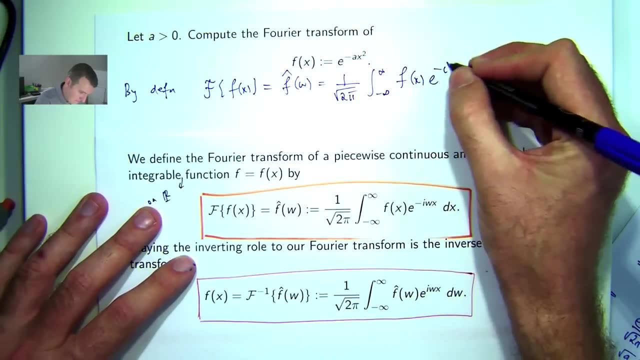 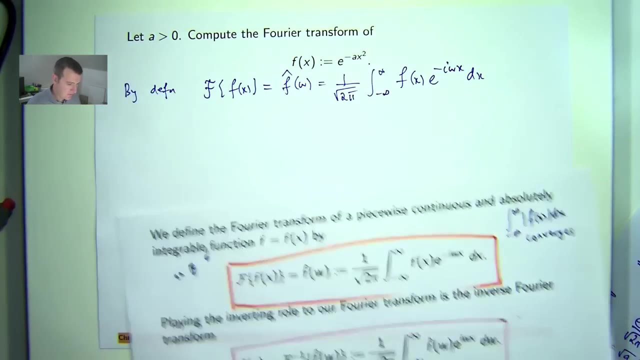 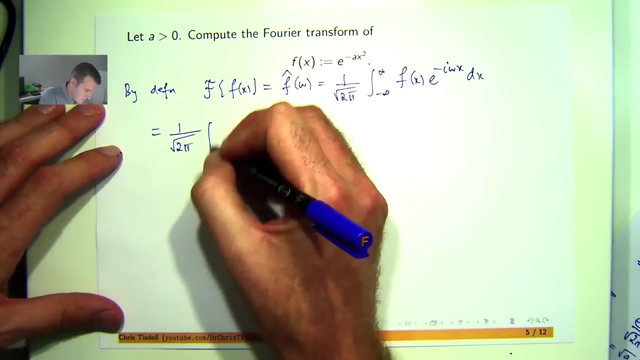 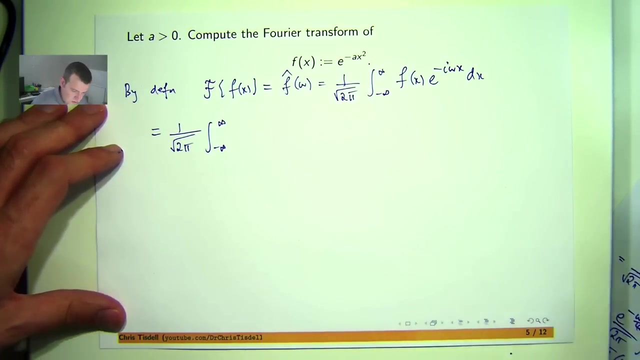 representation. Okay, And so let's replace f of x with this, and then we'll try to knock over the integral. Okay, so this is also an exponential function. so what I can do is team that up with the existing exponential function. 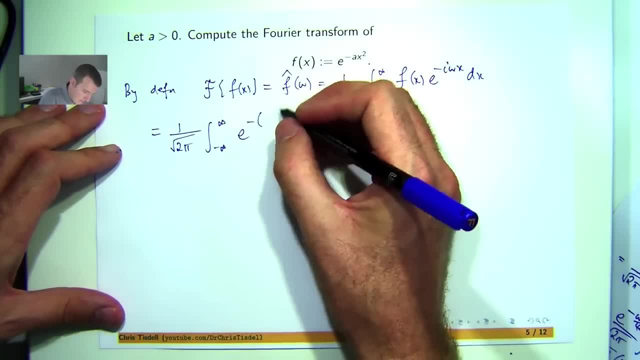 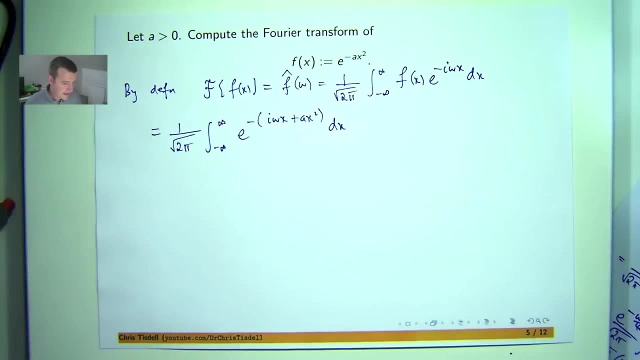 Okay, And I'll get the following: Okay, Now, how do I evaluate this integral? It's difficult because of the x squared up there. Okay, But what I'm going to do is complete the square in x and then that's actually going to simplify. 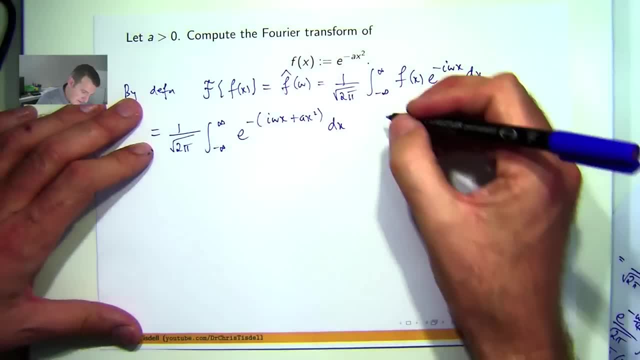 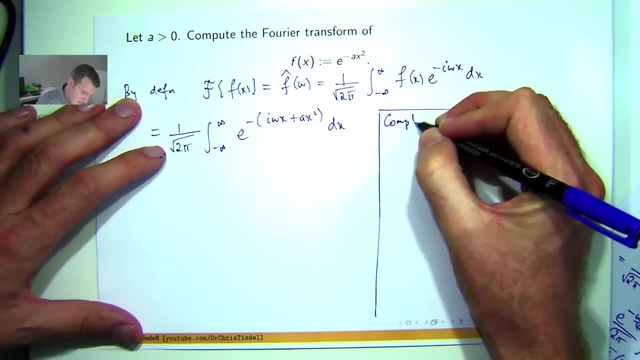 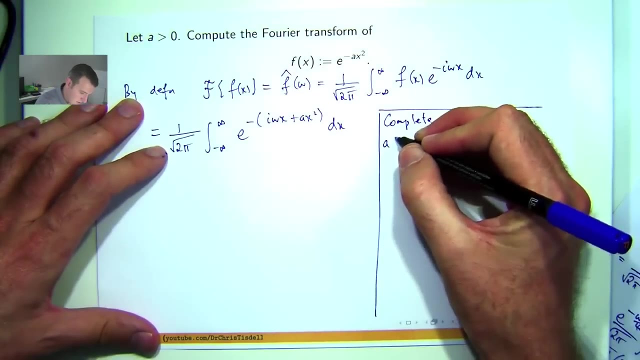 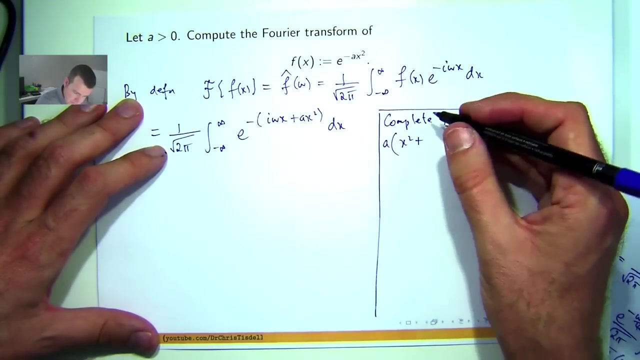 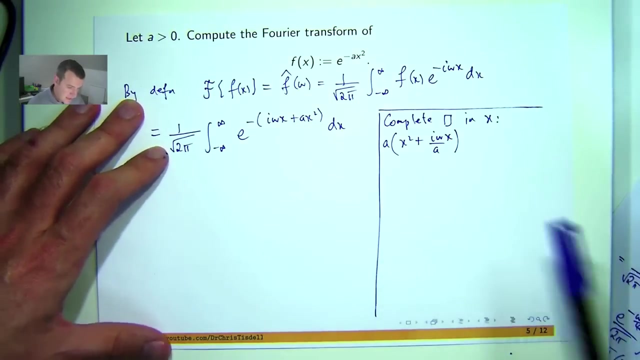 things quite a lot, Okay, So. So I'm going to complete the square in x, Okay. so essentially, I've got something like the following in the brackets here: Okay, managing the a away. So take half the coefficient of x, square it, add it and take it away. 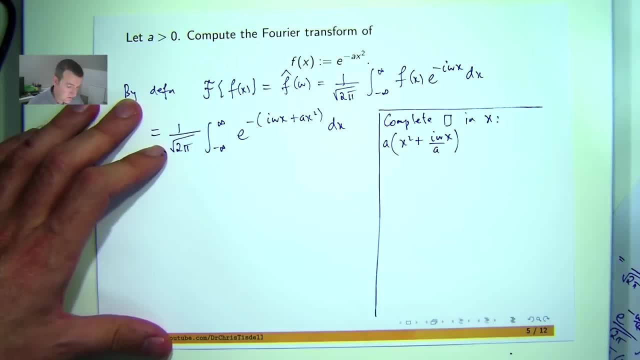 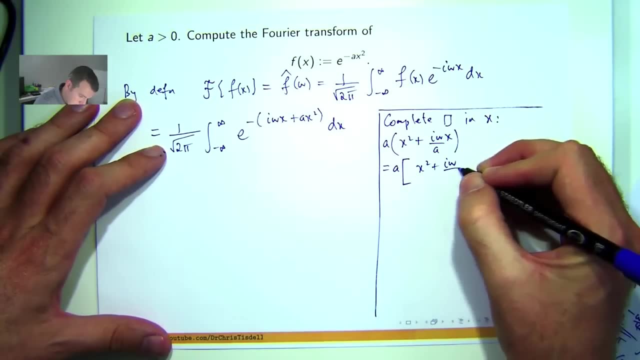 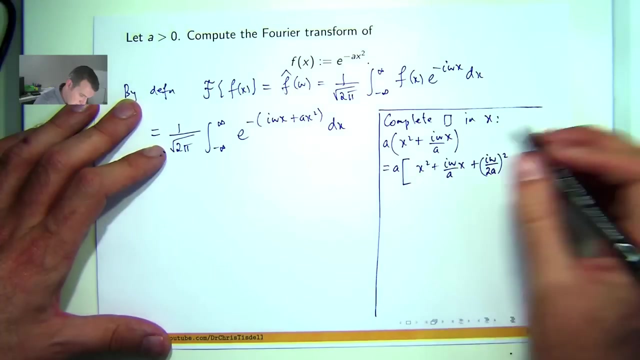 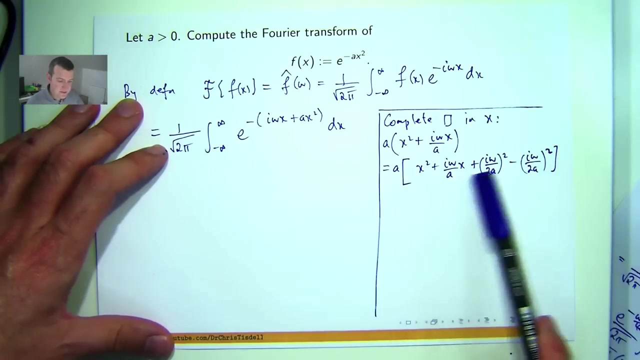 Okay, So, I've got something like this. Okay, So I've got something like this. I've got something like this here. Okay, now these three terms are a perfect square, So I can factor those. It's a Superb. 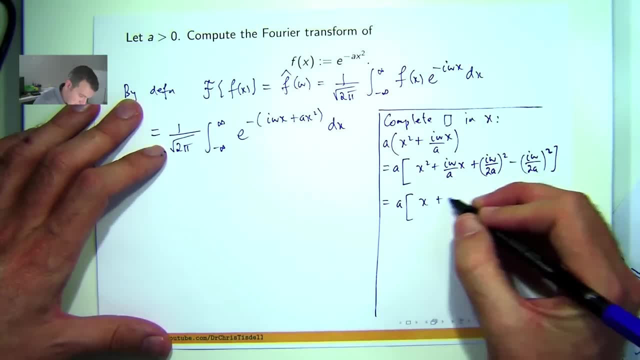 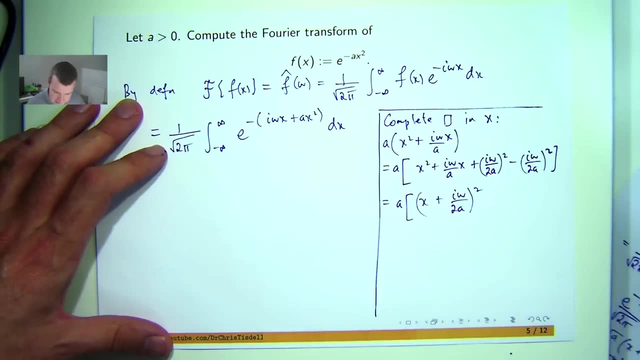 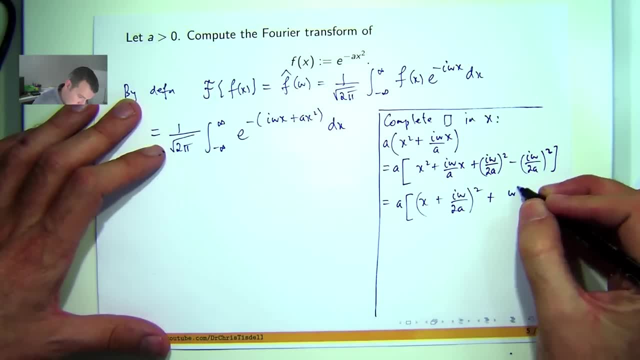 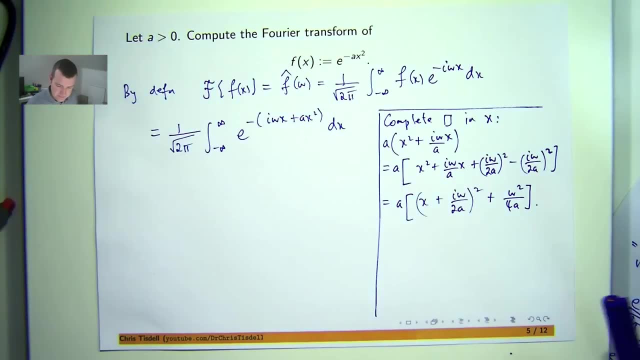 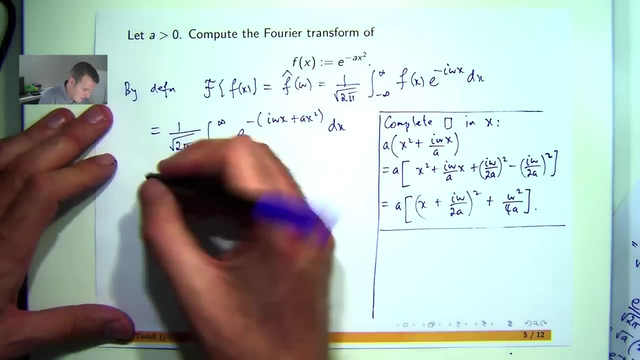 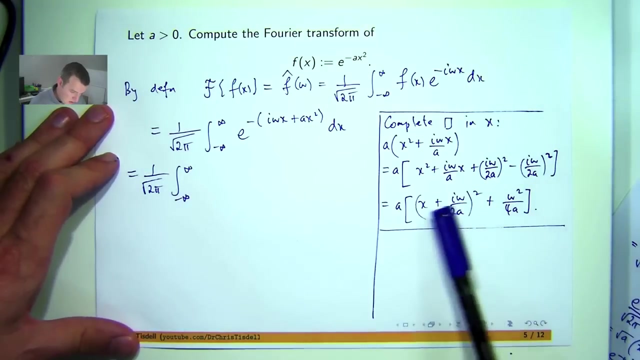 get something like the following: okay, Alright, let's put that back into here and see if that really does simplify our situation. Okay, so e to the negative of that. well, the x, remember, we're integrating with respect to x here. the x's are here. that's got nothing to do with x, so I can break it up into something. 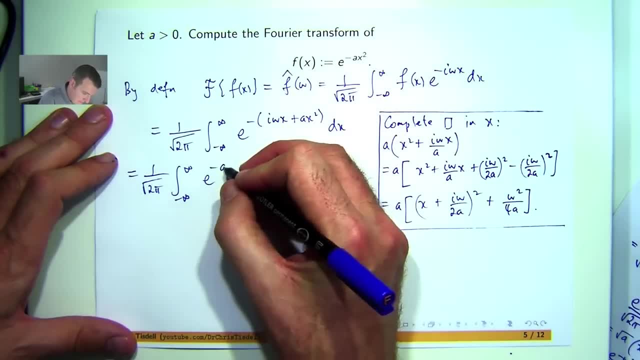 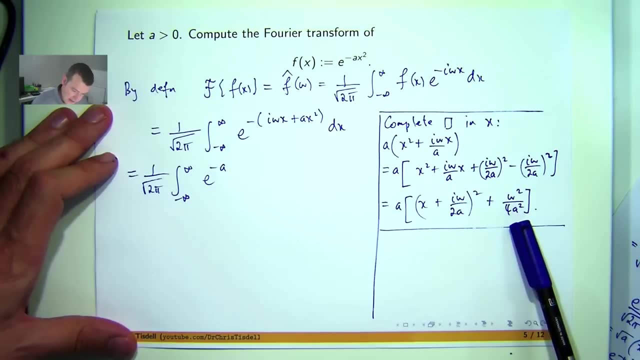 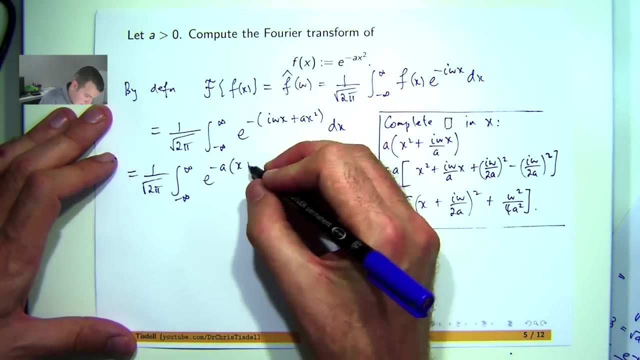 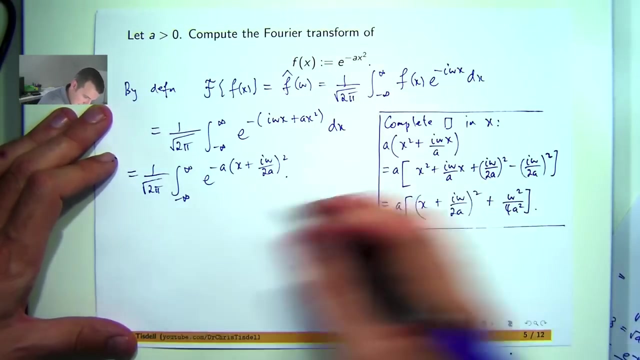 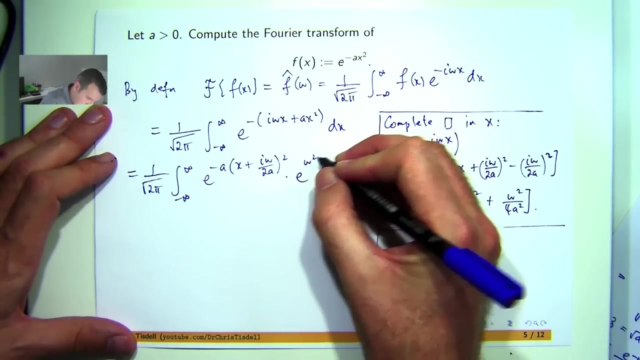 like the following: ah, sorry, it should be a square down there. okay, alright, don't forget that. it should be a square down there. Okay, So times okay. so the a will cancel with that a and I'll get the following. 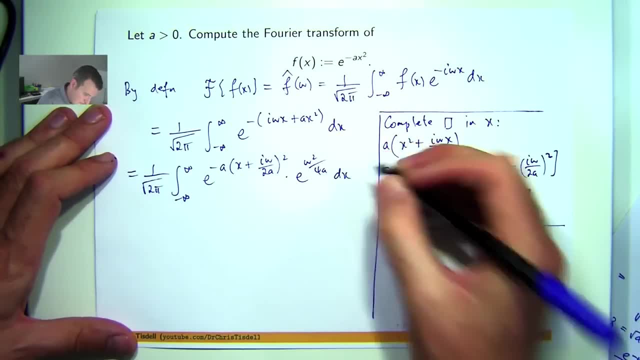 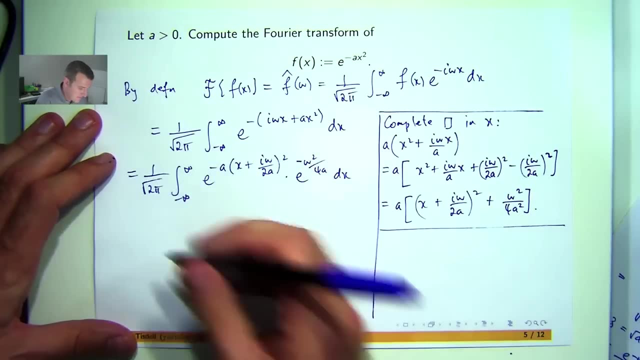 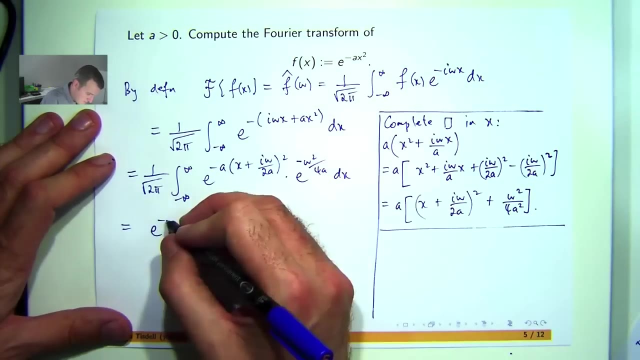 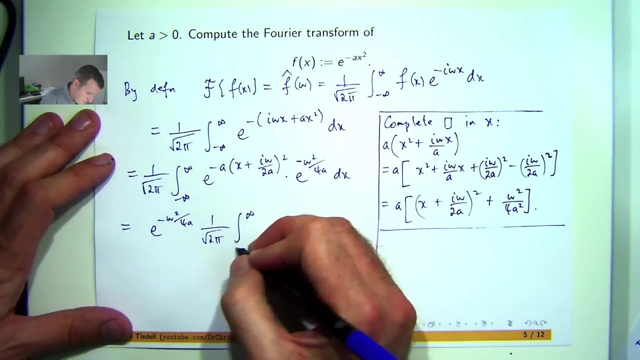 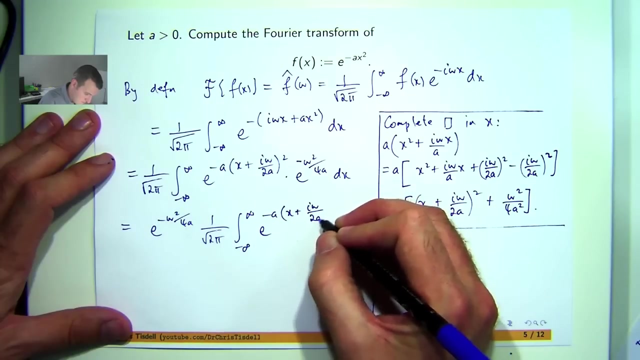 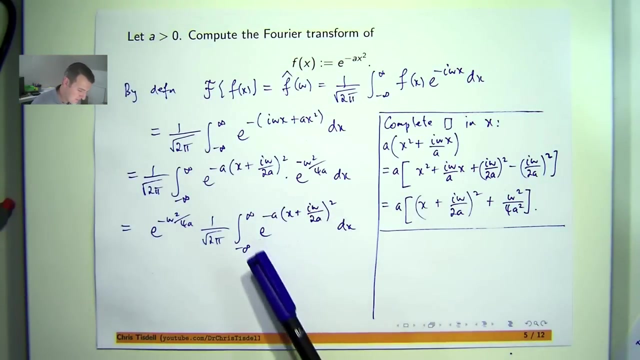 Now, this has nothing to do with x, so I can push that. sorry, I've got the minus sign, so I can push that out the front. Okay, now the question is: how do I evaluate this? Now, it's an improper integral. 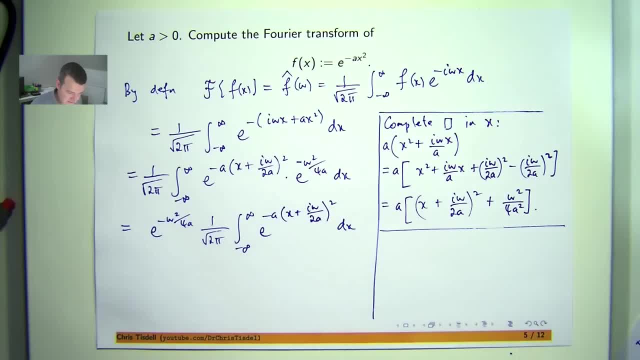 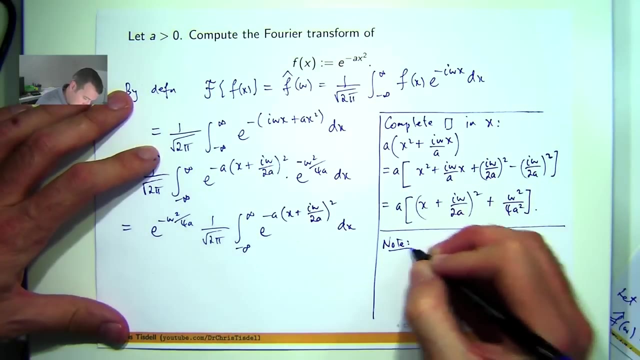 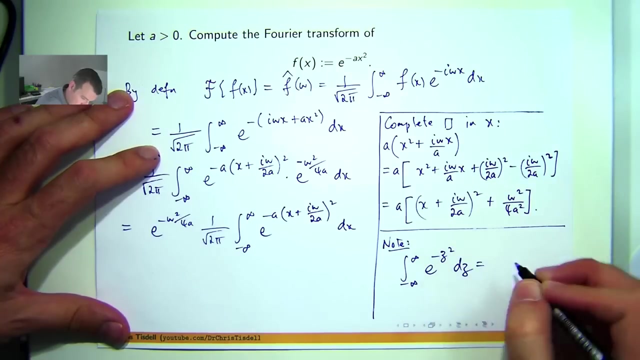 And it's e to the negative, I guess, of something squared. essentially, Now, this almost looks like an error function, which is a special function used in applied mathematics. Okay, So at this stage, we know that we know the following: okay, and I've proved this result. 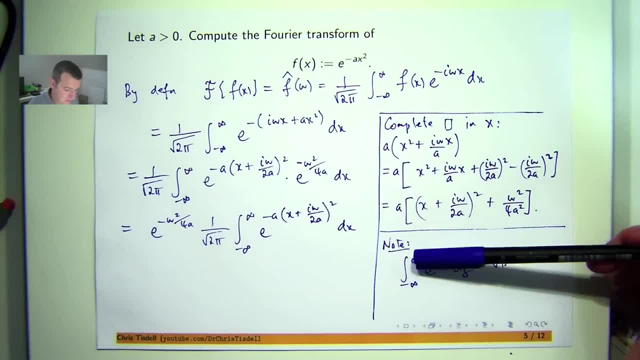 in other videos. In fact, I've proved the result for x. I've proved the result from 0 to positive infinity. is this onto? okay, it's an even integrand. so to go from negative infinity to infinity, you just multiply the result. 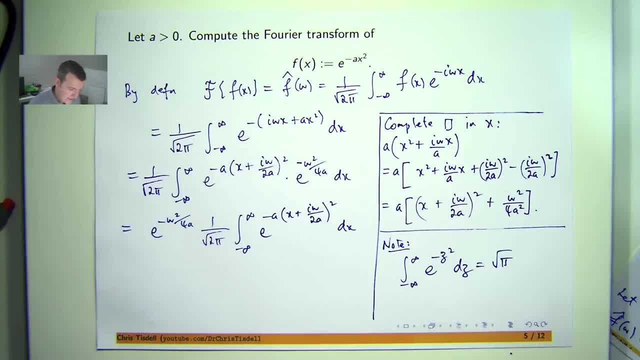 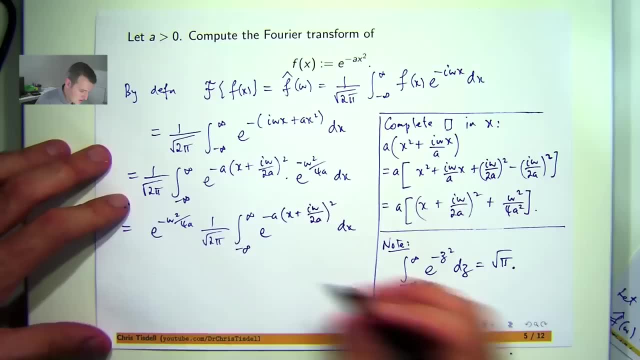 by 2, so that's where the root pi comes from. Okay, so what I'm going to do is make a substitution up here. okay, I want I want that to become a negative z squared. okay, so I'm going to let say, z equal the square root of everything. 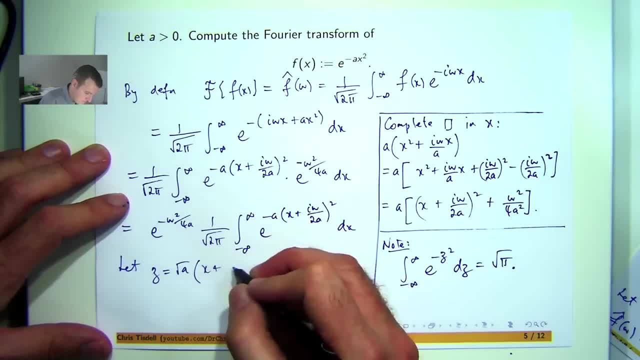 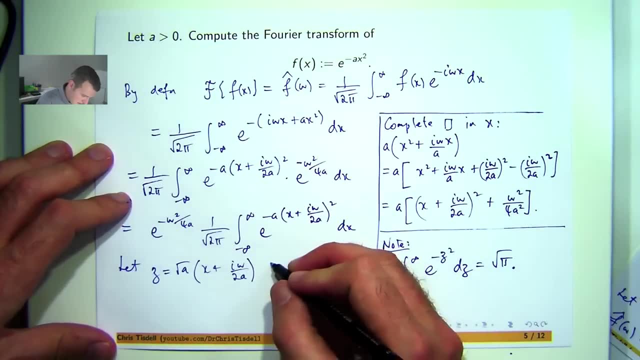 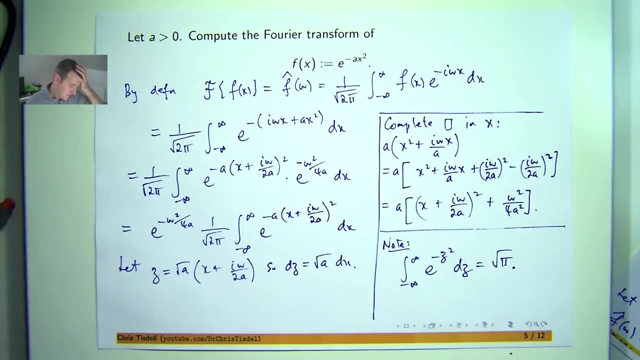 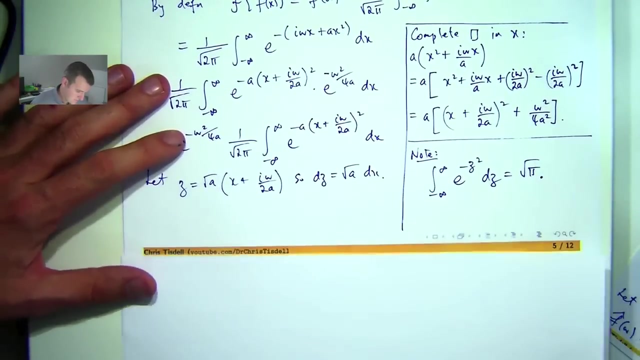 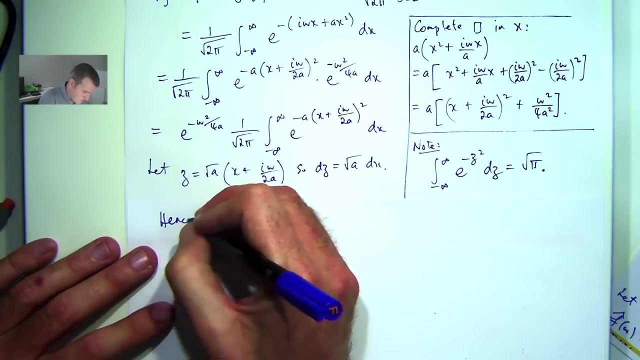 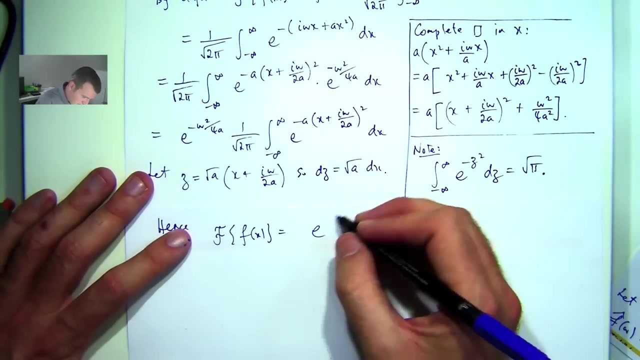 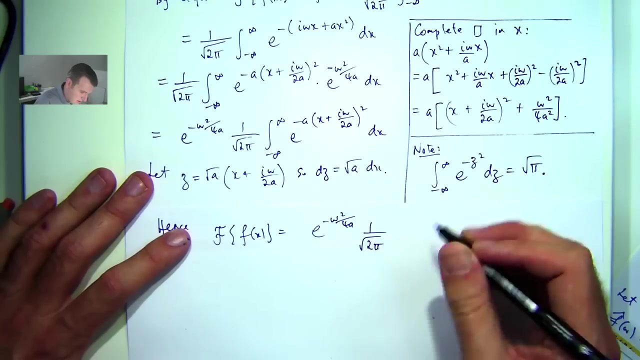 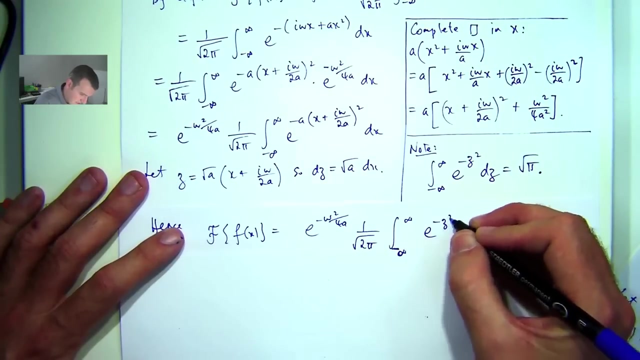 up here. Okay, so if that's the case, then dz is going to be root adx. the limits of integration are going to stay the same, so our transform is going to be something like the following: This won't change, uh-huh. okay, so I'm going to get e to the negative z squared times. 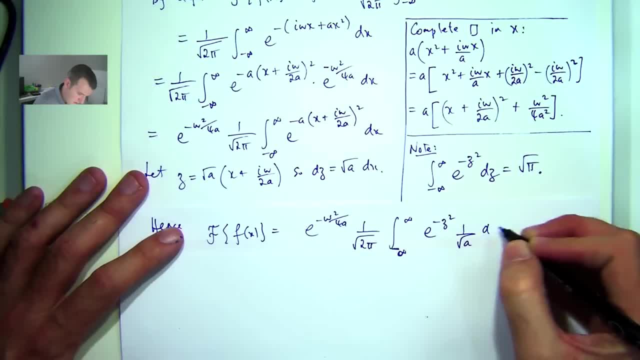 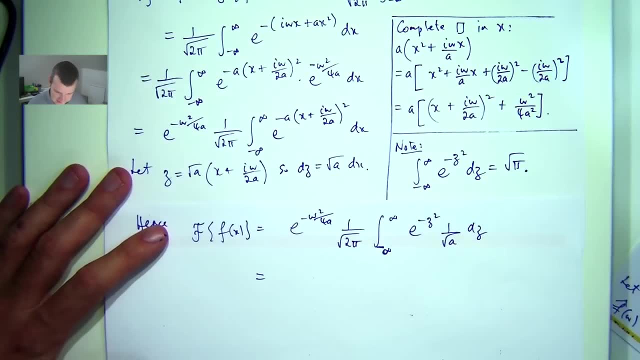 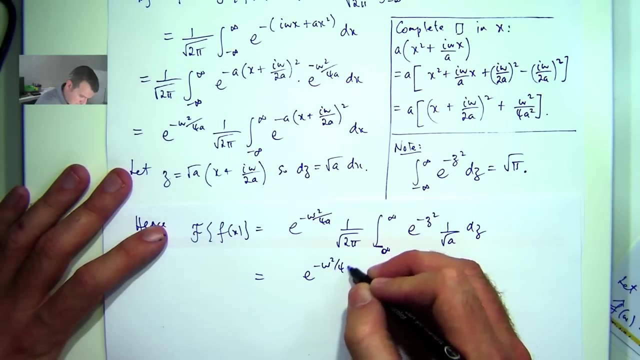 dz over root a. okay, so that can come out the front. and then I'm left, pretty much left with this. okay, Now this: now, if I move that out the front, this from here is just root pi. so the root. 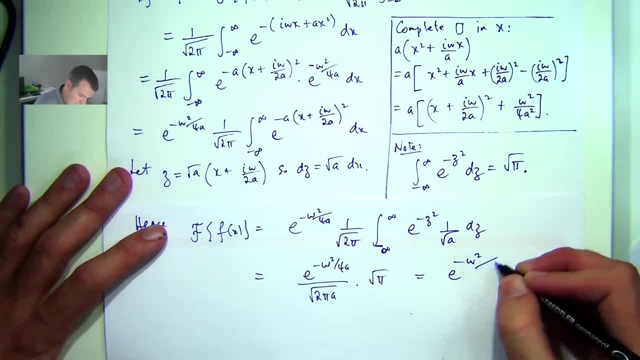 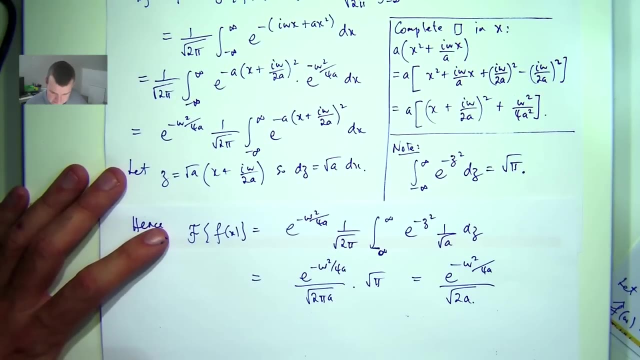 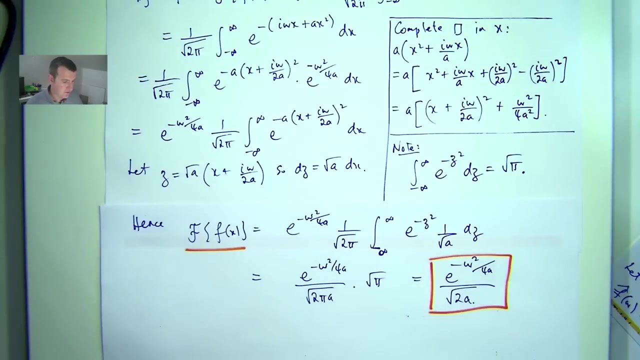 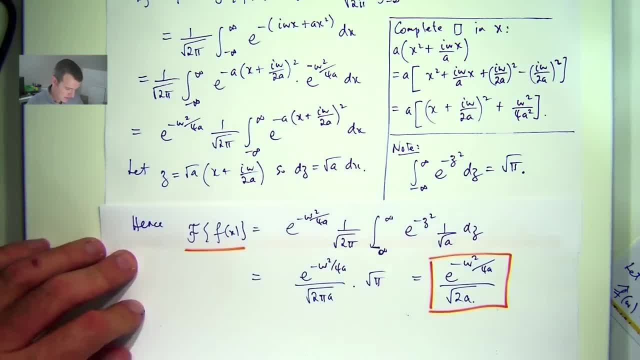 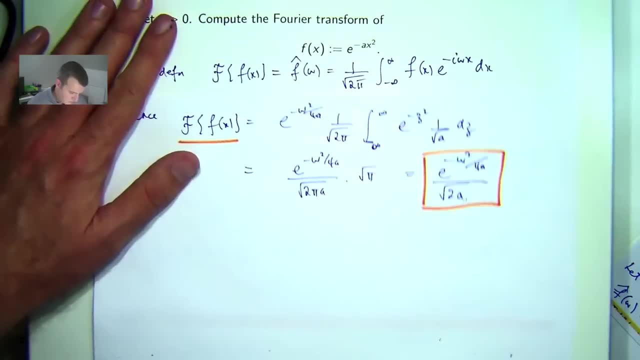 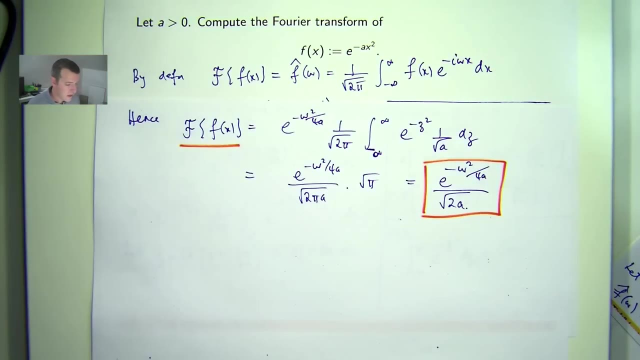 Now, that was a little bit more work than the previous question. Now, um, a good question here is: why. why is this result important? Okay, why is this an important transform? to spend some time learning how to work out. Well, first of all, we want you know. one answer to that is that you know, we want. 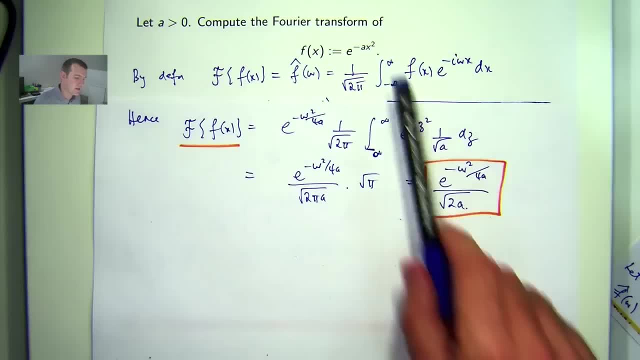 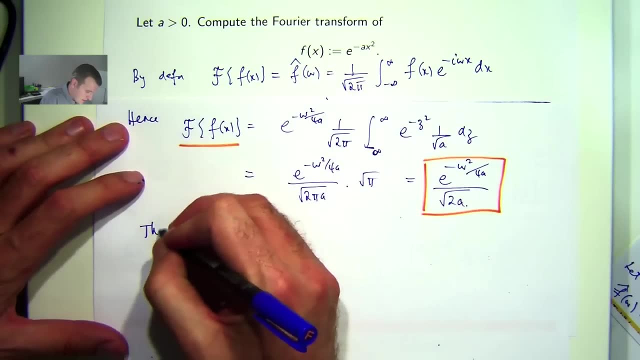 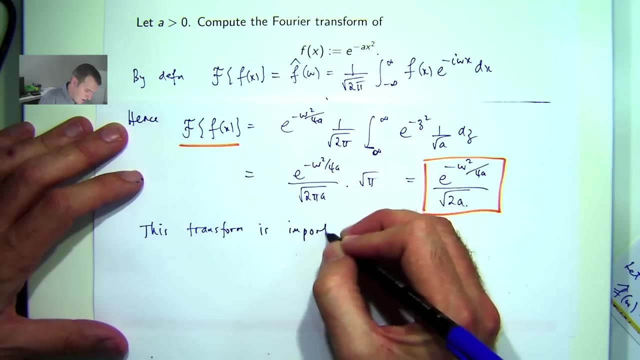 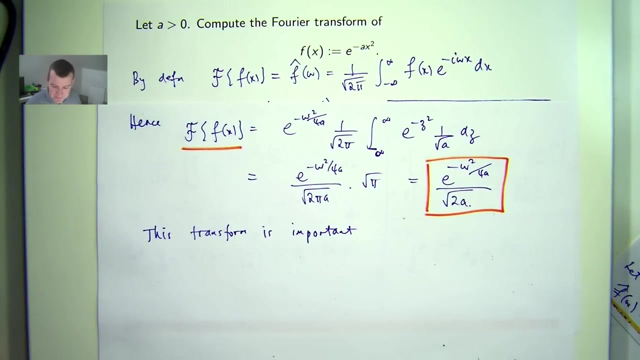 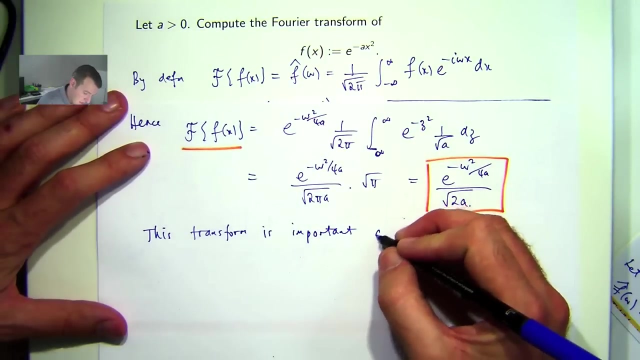 to get familiar with the transform technique. Okay, but why is this particular function important? Well, this particular function is important Because you'll see it when we're solving partial differential equations and, in particular, when we're studying diffusion or heat problems involving PDUs.